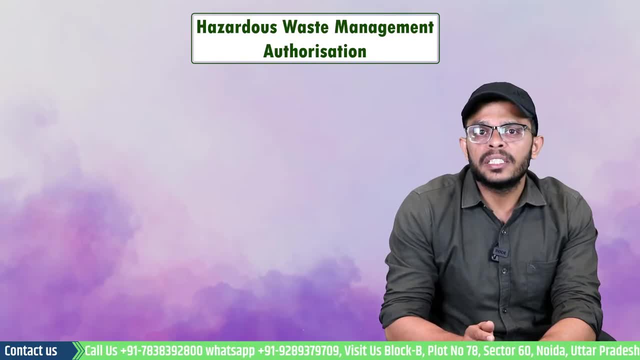 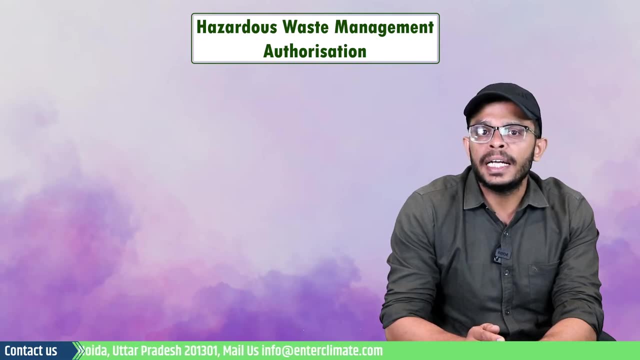 44,000 industries. With this much hazardous waste being produced, the government enacted the Hazardous Waste Management and Handling Rules of 2008, which regulated and ensured proper hazardous waste management and was governed under the Ministry of Environment, Forest and Climate Change. Secondly, the Centre Pollution Control Board and the State Pollution Control Board were 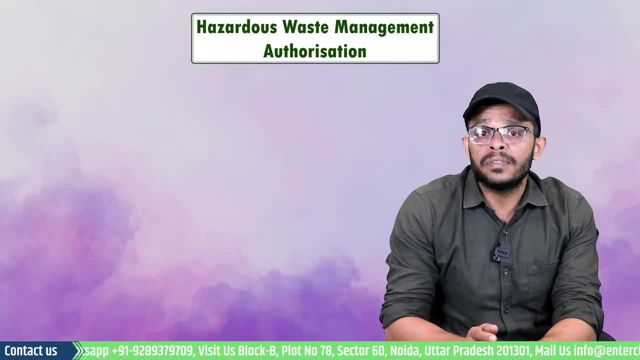 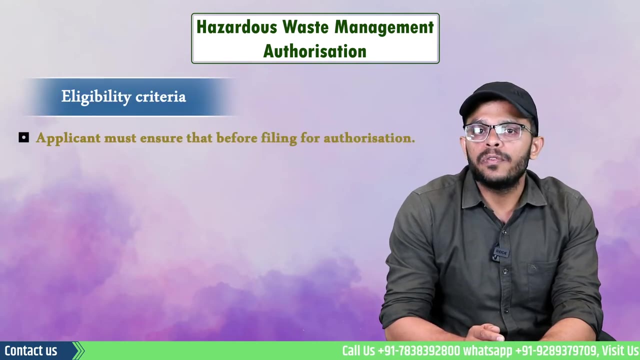 also included. These rules also mandated hazardous waste management in 88 hazardous waste incinerators and around 220 recycling facilities in the country. Let's now discuss the eligibility criteria for setting up a hazardous waste management business. The applicant must ensure that, before filing for authorization, 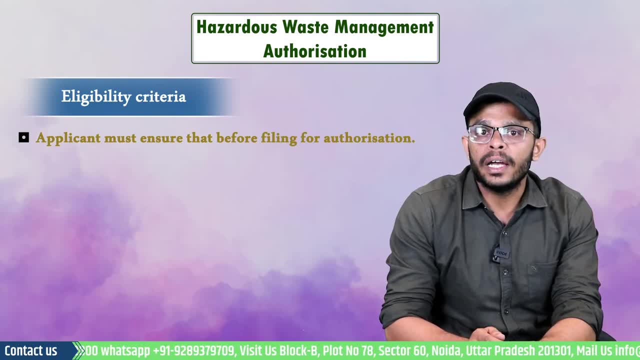 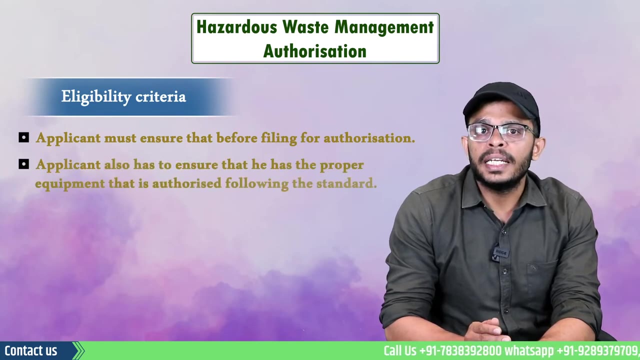 the hazardous waste is properly collected, stored, treated and recycled in the facility which fulfils the provisions mandated under the Hazardous Waste Management Rules of 2016.. Apart from the proper premises and space, in accordance with the law, the applicant also has to ensure that he has proper equipment. 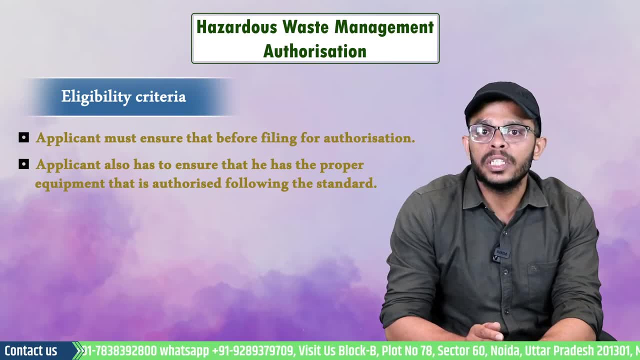 that are authorized following the standard operating procedures or other regulations specified by the Centre Pollution Control Board for properly recycling and managing hazardous waste. Furthermore, the unit requires a skilled workforce to handle hazardous waste properly and lessen the environmental damage it can cause, rather than increase it. 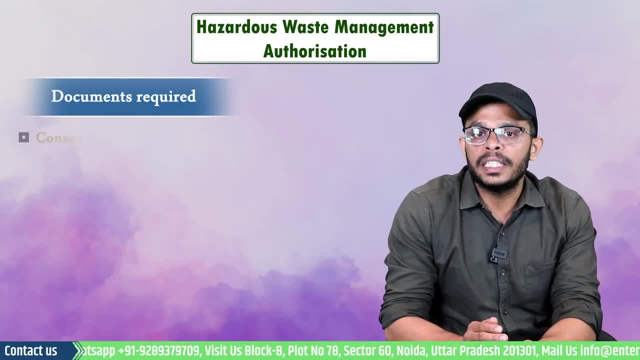 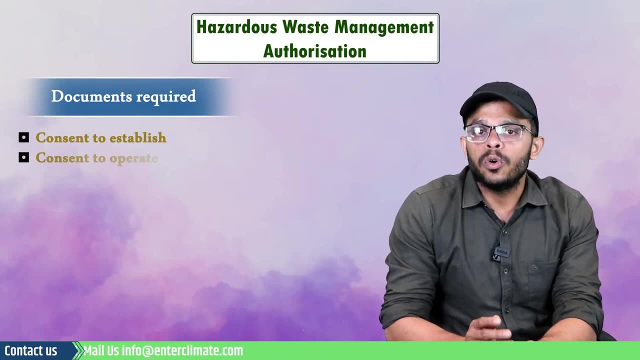 So the documents required for Hazardous Waste Management authorization will be the consent to establish, which will be granted by the concerned State Pollution Control Board, the consent to operate granted by the State Pollution Control Board, GST certificate, rent lease or any other proof of ownership. 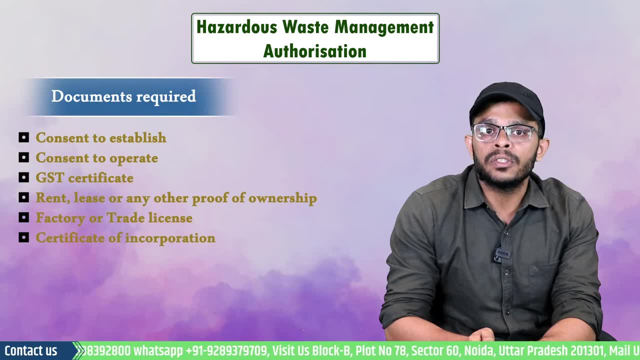 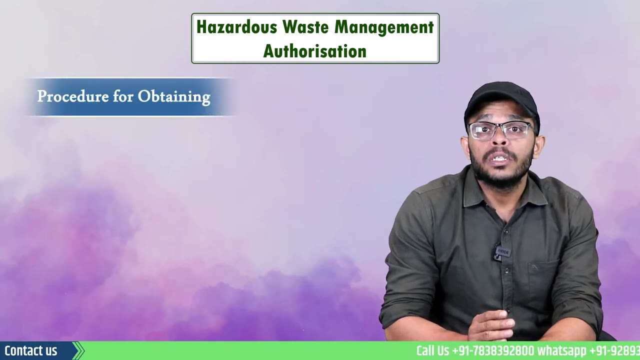 or trade license, certificate of incorporation in case of the company, or an LLP layout plan, Aadhaar card copy, PAN card copy and the electricity bill. Let's now understand the procedure for obtaining Hazardous Waste Management authorization. So the applicant has to fill Form 1 as per Rule 6 of the Hazardous and Other Waste. 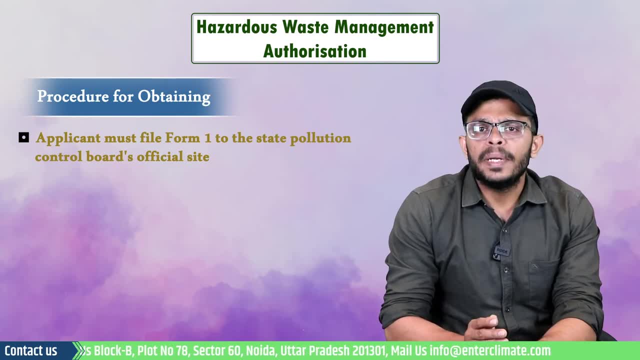 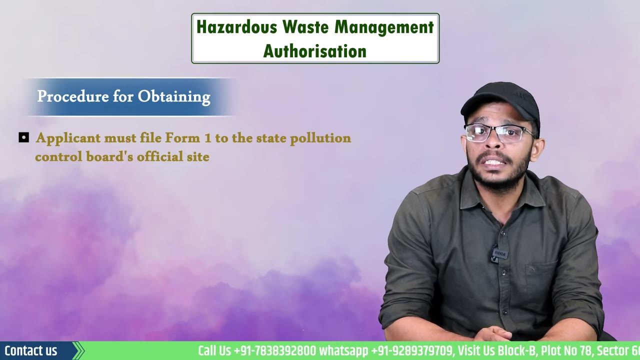 Management and Transboundary Movement Rules of 2016.. The applicant must file this form and submit it to the Board's official site after creating a registration ID. This form is to be submitted with the required documents. After receiving the application, the State Pollution Control Board conducts a proper inquiry.